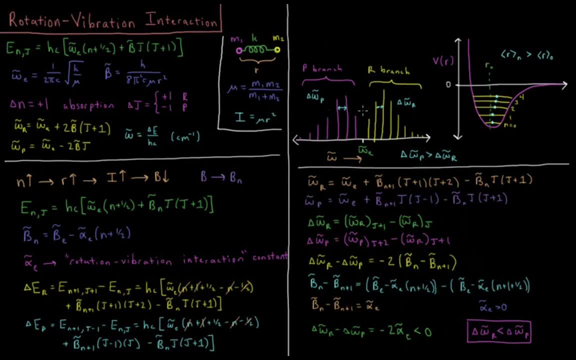 branch, And if we have a perfectly harmonic oscillator and a perfectly rigid rotor, this should not be the case. So this video will explain why these spacings are not equal and what the physical reason for that is. So we'll remind ourselves of our diatomic molecule. 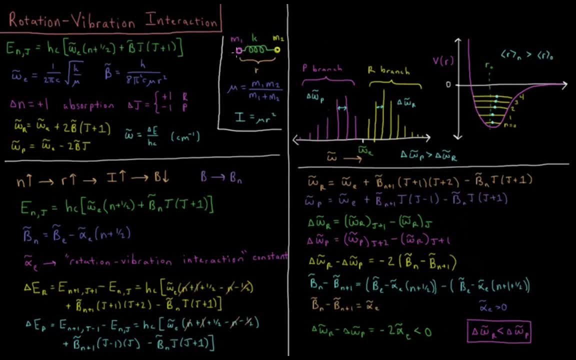 model Two: atoms of mass one and mass two, connected by a covalent bond with a spring constant. k potential equals one half k x squared. We have a bond length of R and we have a reduced mass of m1 times m2 over m1 plus m2.. Momentum, inertia, resistance to 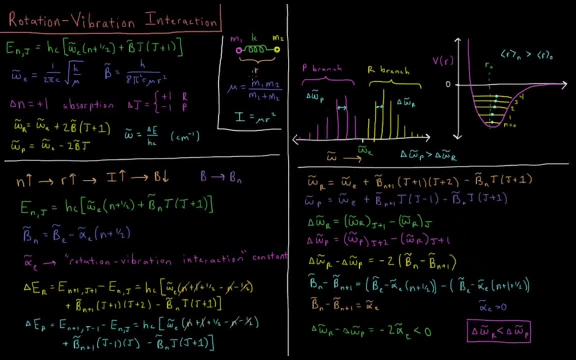 angular acceleration equals mu times R squared The energies of our row. vibrational energy levels as a function of quantum numbers n and j, which are both integers, starting at zero going up to infinity, equals hc Planck's constant times. speed of light in centimeters. 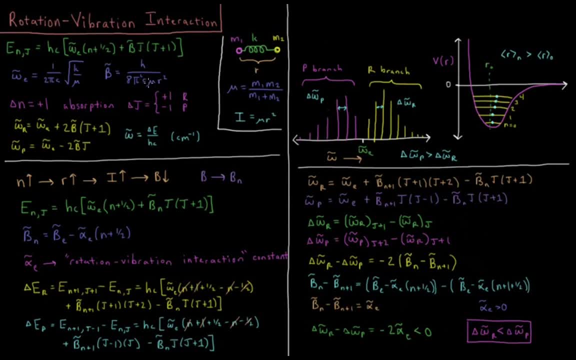 per second. Speed of light c will always be in centimeters per second in this video Times. omega e times n plus one. half plus b-bar. times j times j plus one. Omega e is the vibrational constant which is one over two pi c, square root of spring constant divided by reduced mass, b-bar. 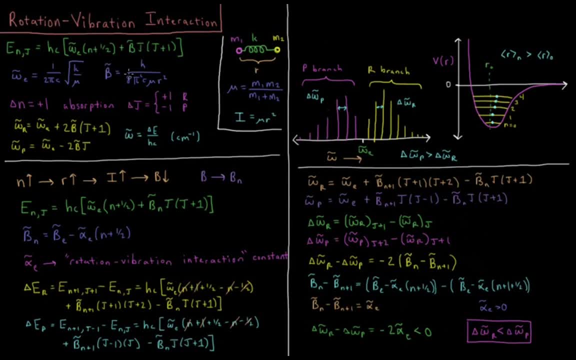 the rotational constant is equal to Planck's constant divided by eight pi squared. speed of light times. reduced mass times: r squared. The right-hand side of the graph shows that the energy Celsius orufil is less than or equal to the energy P. Our selection rule for the row vibrational spectrum was that delta n. 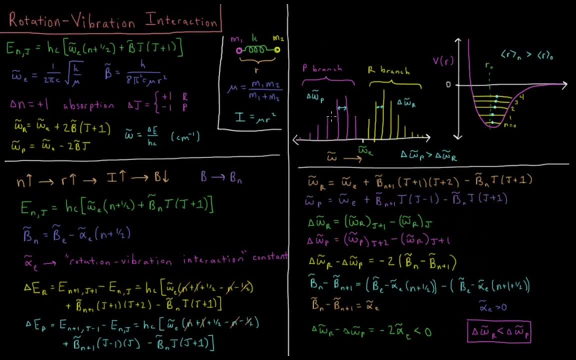 equals plus one. It is an absorption. We are absorbing a photon with some amount of energy equal to our energy jump. Delta j equals plus or minus one. Plus one is more energy going up to our branch. minus one is less energy going down to the P branch. The inverse wavelength. so the in-wave numbers is the strength. The frequency is no longer so. the wave is as high at the edge as it is at the edge. The energy is dictated by the frequency. We have all the seniors and seniors. The reason that the index is not a constant is because of the stress, The 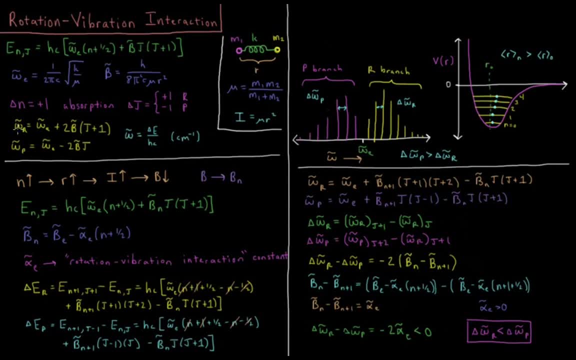 numbers. one over the wavelength of our photon for the R branch is the rotational constant plus two, sorry, vibrational constant plus two times rotational constant, times quantum number J plus one starting at zero. For the P branch, the inverse wavelength of our photon is the vibrational constant minus. 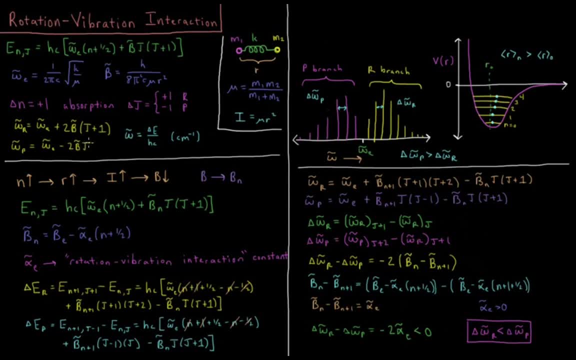 two times rotational constant times, quantum number J, starting at J, equals one. Okay, so we end there. omega bar equals delta E over hc units of wave numbers. Okay, so what's going to go on here that's going to cause a deviation from this behavior? 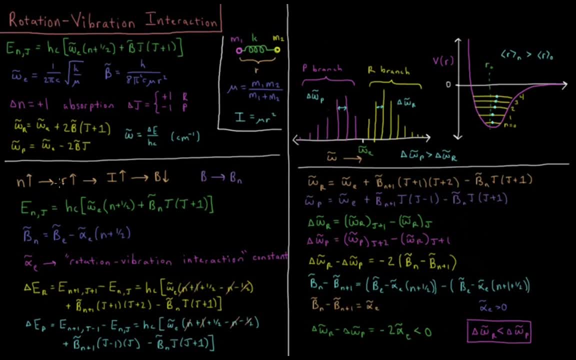 So as the vibrational quantum number goes up, our R, our bond length, is not going to be constant. In a perfectly harmonic oscillator, our average bond length, R naught, would stay the same at every single vibrational level. But in fact our P branch would stay the same at every single vibrational level. 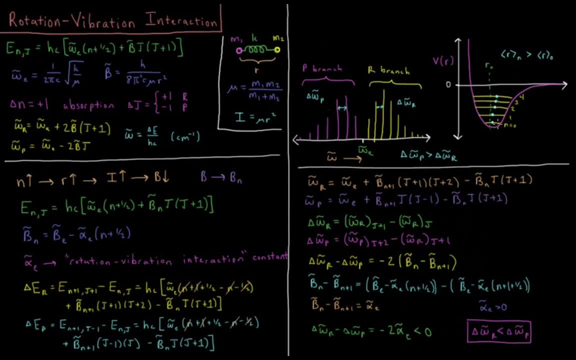 Our potential energy surface is not perfectly harmonic. In fact, it's anharmonic. Specifically, it's anharmonic towards an increasing bond length. This wall is very hard, this tail is very soft, so the bond prefers to stretch as we get to higher and higher energy levels. 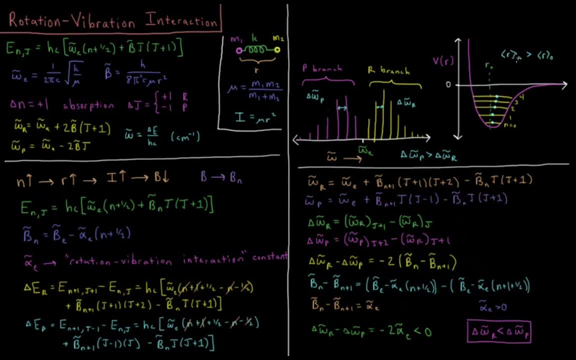 So what happens is our bond length for n greater than zero is greater than our bond length for n equals zero And if you'll notice, So, as our vibrational quantum number goes up, bond length goes up. That means moment of inertia goes up because it's mu R squared. 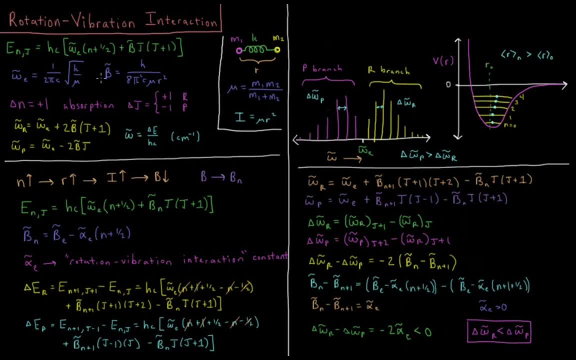 And I is in the denominator mu R squared of B bar. So B is going to go down. So what we do here is we build a model where B is a function of our vibrational quantum number. The rotational constant changes as we go up in vibrational quanta. 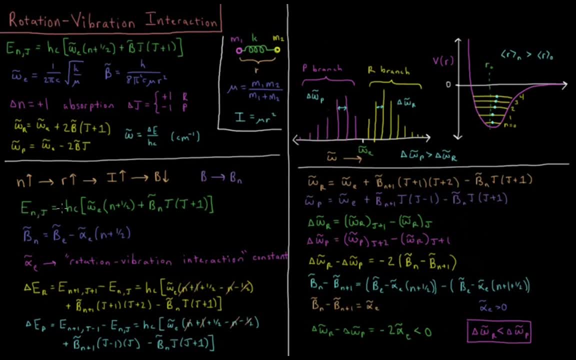 Okay, So now E of n and j equals hc. omega e times n plus one half, plus B bar n times j times j plus one. B bar n is equal to B bar e, our equilibrium value of B bar, our average bond length at. 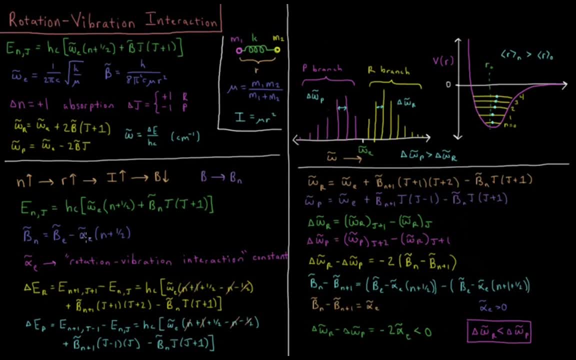 the minimum of this potential minus alpha e, times n plus one half. So alpha e is called the rotation vibration interaction. So alpha e is going to serve to decrease the value of our rotational constant as we go up in vibrational quantum number. So now, using this model, we can calculate the change in energy in the R branch and in. 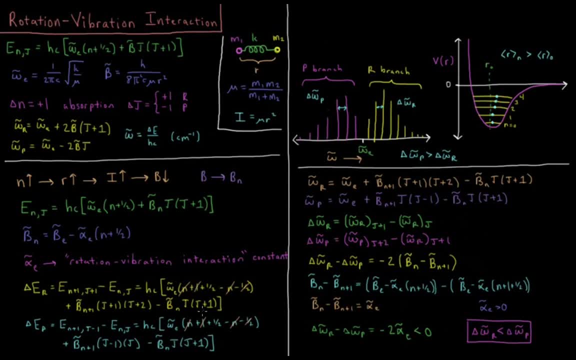 the P branch And we're going to go through a bunch of algebra there And that delta e is going to end up giving us our frequency of our light that we absorb in the R branch and the P branch. So that's going to be omega e plus B, bar n plus one j plus one times j plus two minus. 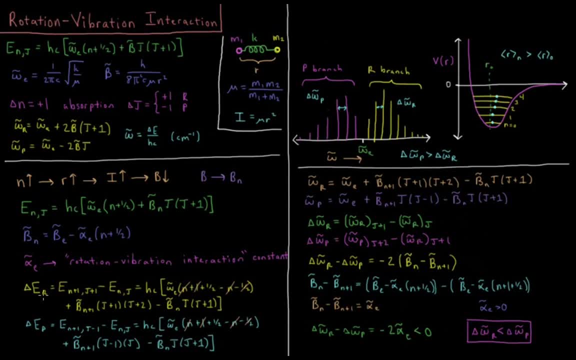 B bar n? j times j plus one, because in the R branch we're going from n plus one- j plus one- to n? j, or, sorry, from n? j to n plus one, j plus one. In the P branch we're going from n? j to n plus one, j minus one. 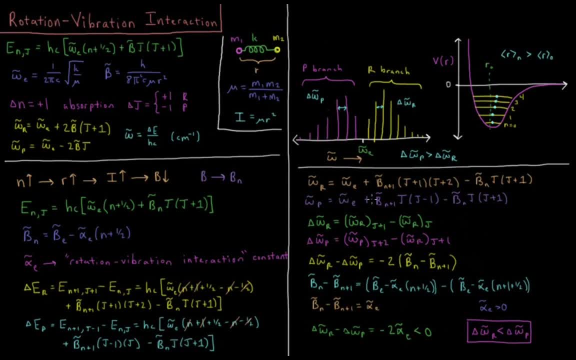 That gives us a frequency of absorption of omega e plus B bar n plus one j times j plus one, j times j minus one minus B bar n j times j plus one. So now we'll look at the difference between two subsequent frequency transitions. So the difference between this peak and this peak, versus this peak and that peak, this 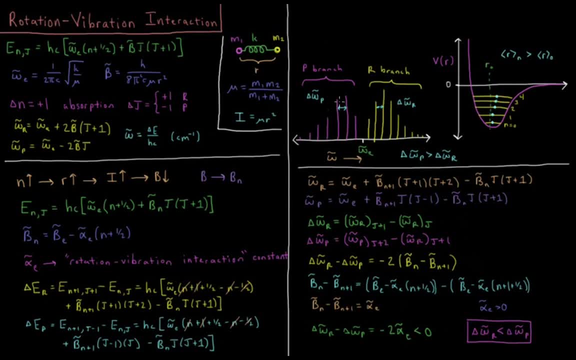 one and this one versus this one and that one, et cetera. So we'll call this delta omega R. The difference between these two peaks is omega R of j plus one minus omega R of j. Delta omega P is going to equal omega P of j plus two minus omega. this should be omega. 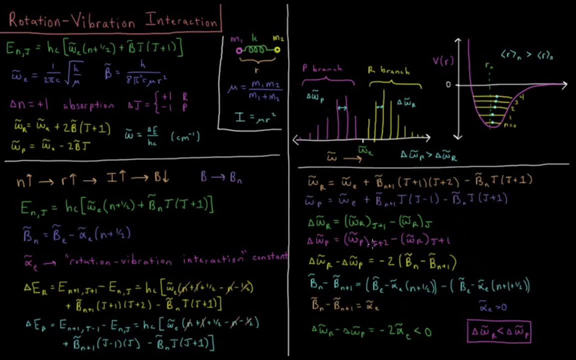 P of j plus one. So we have j plus two and j plus one here, because in this one j goes up, in this one j goes down. So we are comparing equivalent peaks there. So when we compute these two numbers, we have delta omega R minus delta omega P. once you. 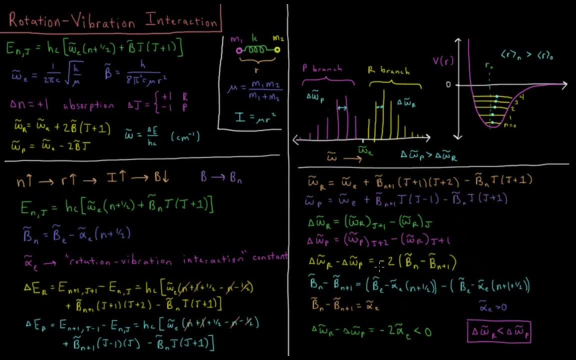 work through all the algebra, I'll save you the time. equals minus two times B bar n minus B bar n plus one. So this is going to equal this B bar n minus B bar n plus one. We get from our model for what B bar n is: B bar e minus alpha bar e n plus one half. 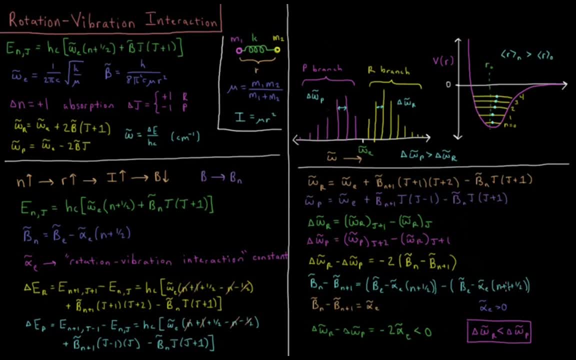 minus B bar e, minus alpha e, n plus one plus one half. So the difference between these two rotational constants is just alpha e. So substituting it up here, we have that the difference between subsequent peaks in the R branch minus that difference in the P branch is minus two alpha e. 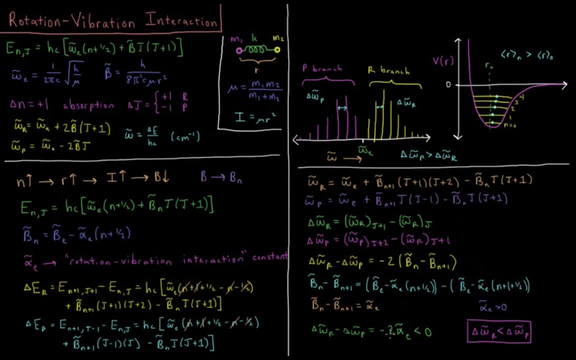 Alpha e is a constant which is greater than or equal to zero, So that means that minus two alpha e is less than zero. If delta omega R minus delta omega P is less than zero, that means that delta omega R, the difference in spacing in the R branch, is less than delta omega P, or less than delta. 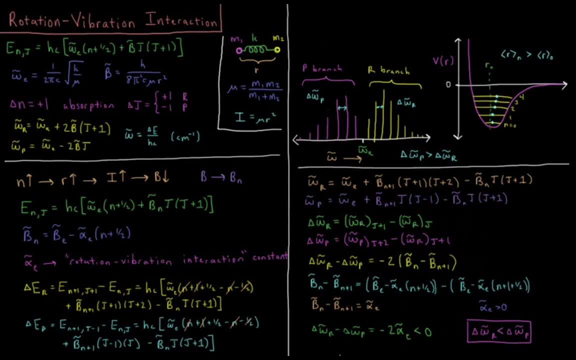 omega P, the difference in spacing in the p-branch. So notice here: according to our model, the difference in this spacing is entirely proportional, directly proportional to alpha e, the rotation vibration interaction constant. This is a measure of the anharmonicity of our vibrational potential energy. 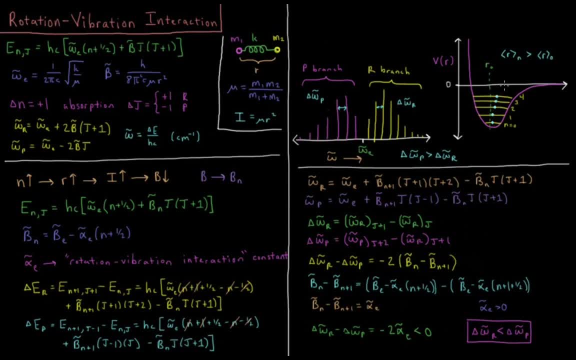 surface. So as the vibrational, as the vibration gets more anharmonic, this will get bigger. there will be a more pronounced difference in spacing between the r-branch and the p-branch and as they get equal to one another, as it becomes more perfectly harmonic, these two become equal and 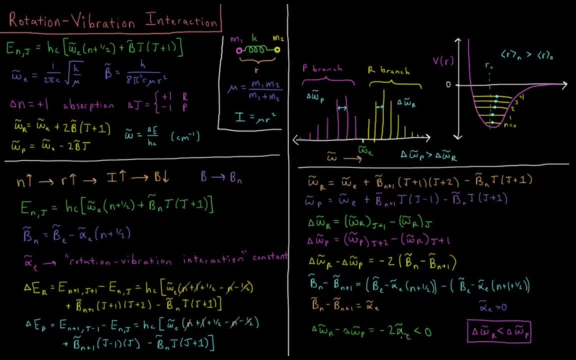 correspond to our earlier models. So this rotation vibration interaction constant with a vibrationally dependent rotational constant due to the anharmonicity and different bond lengths at different vibrational energy levels, does a good job of predicting this difference in energy between two different vibrational energy levels. So this is a good example of how we can predict. 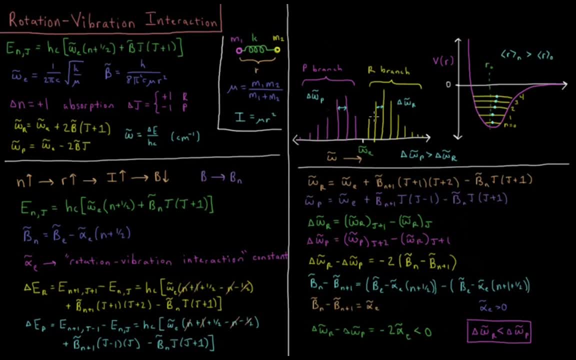 peaks in our p-branch and our r-branch of our row vibrational spectrum.